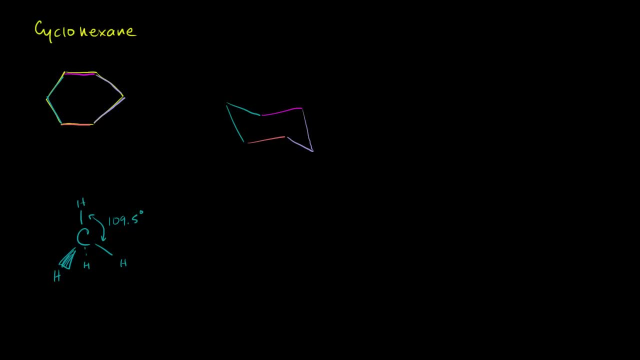 And this way that I've drawn the cyclohexane is called a chair configuration And it might be obvious. It looks like a chair. That's the back of the chair. This is where you would sit down on the chair and I guess 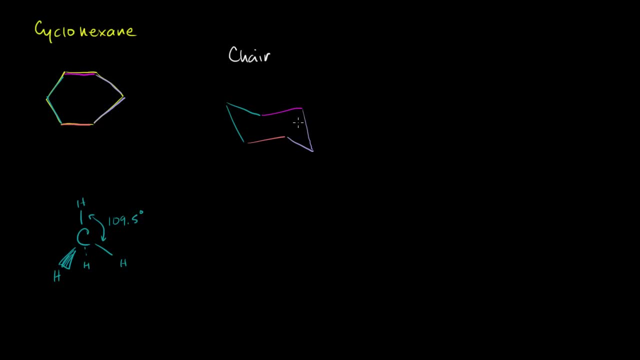 the back of your calves would go down Right. If you go against here. your knees would sit on it someplace like that. That's called the chair configuration. Now, another configuration that it could be in is called the boat configuration, And so if I were to put this exact one in the boat, 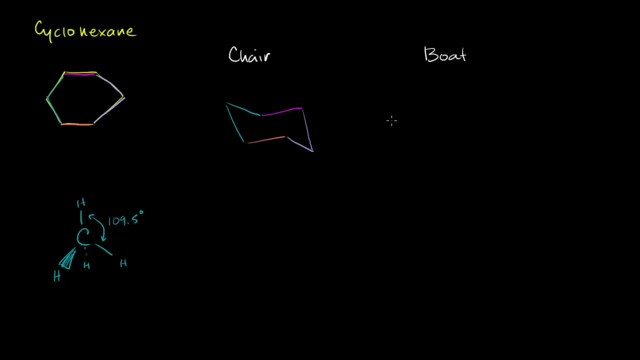 configuration. if I take it from a slightly different perspective, if I'm looking at it kind of head on, it would look something like this: In the boat configuration it would look like this: And I want to use the purple. It would look like that. 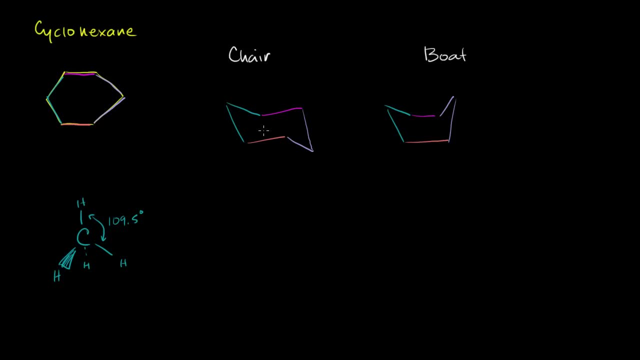 Now, the first thing you're probably saying is: Sal, you said that the reason why it looks like this is because carbon likes to form these kind of tetrahedral or this tripod-shaped bonds. I don't see the tripod-shaped bonds either here or here. 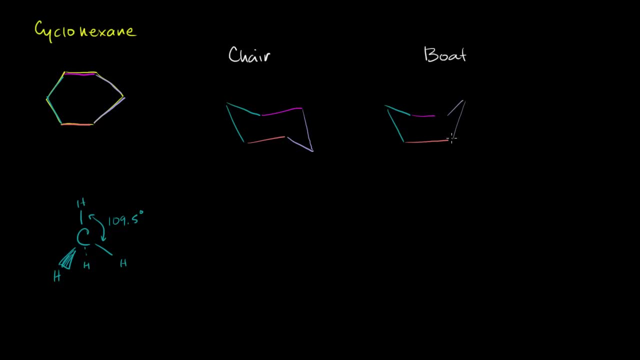 Let me draw that boat a little bit, at least this end of the boat a little bit better. There you go And you say: well, I don't see that tripod. There's a tripod shape over there, And to see the tripod shape you just have to. 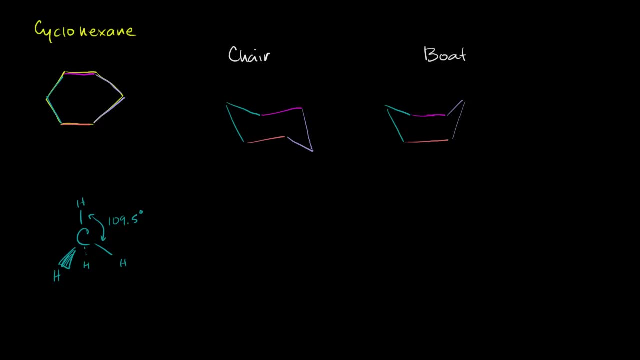 draw the hydrogens. So let me draw some hydrogens here. So let me draw a hydrogen here that will go straight down, like this: a hydrogen that goes straight down over here, a hydrogen that goes straight up over here, straight up over here, straight down over here, straight up over there. 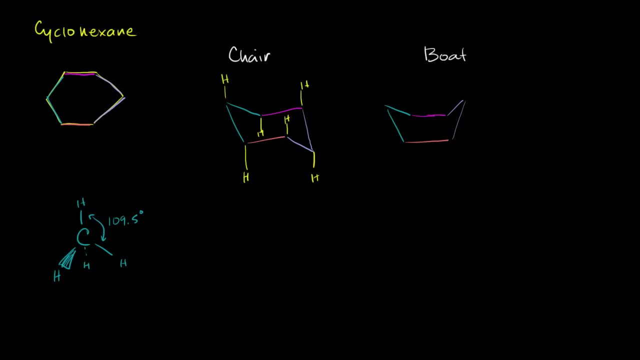 I've now drawn one hydrogen on every carbon. and now let me draw some hydrogens. Let me draw a hydrogen here that goes straight over here. So a hydrogen there. Let me draw a hydrogen over here that does the same thing. So those guys have their hydrogens. 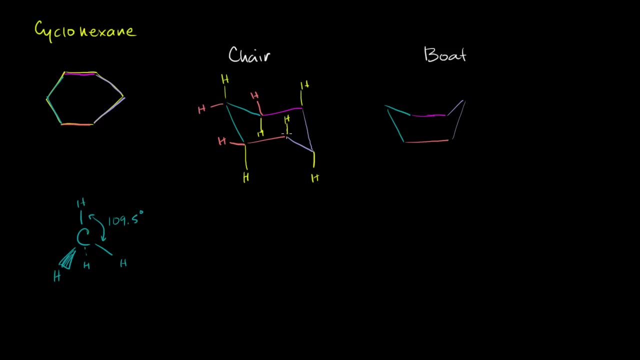 A hydrogen right over here. And then, let's see, this guy needs his hydrogens still, So he'll have a hydrogen that goes down like that and a hydrogen that goes like that, And then this guy will have a hydrogen that goes like that. 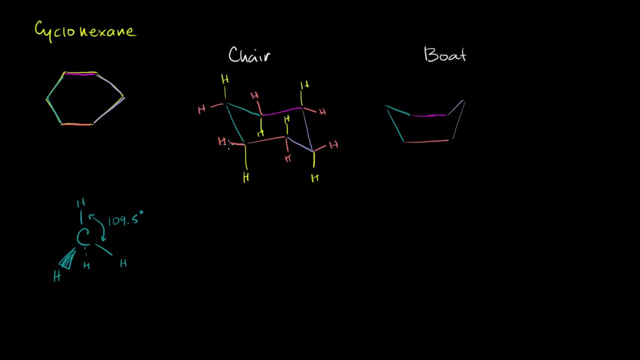 And when you see it like this, if you look at any one carbon on this molecule, you can see that it's forming the same tetrahedral shape, that it has a tripod at every one. Over here you have that close to roughly 109, 110 degree. 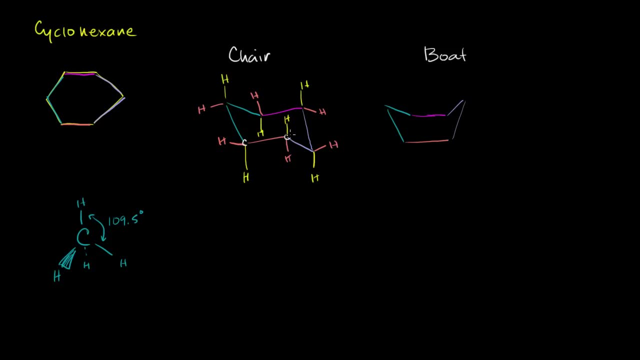 angle between each of the constituents that are bonding to the carbon. Now I've drawn the different hydrogens that are coming off of these carbons in different colors and I've done it for a purpose: The ones that are going straight up or straight down. 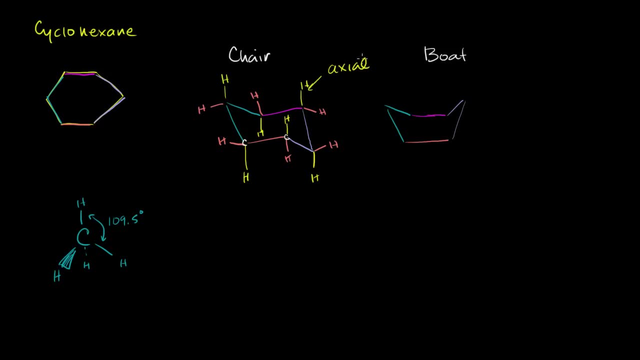 we call those axial hydrogens And the ones I drew in orange that are kind of going to the side in some level. we call these equatorial. These are equatorial And they're called equatorial because they're the same thing as the hydrogen. 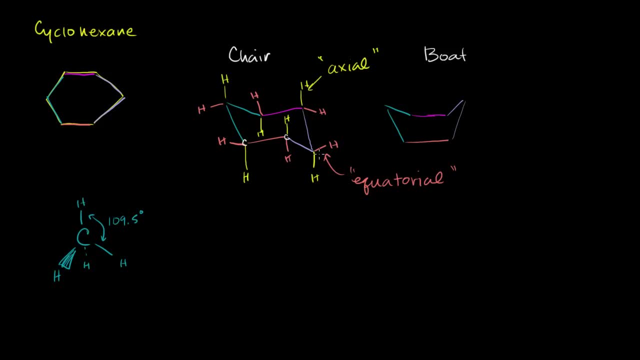 And the reason why it's useful to know that name is when we talk about the different configurations, the different chair and boats. whether something is equatorial or axial can change if this were to flip up or vice versa and things like that, And we'll talk more about that in the next video. 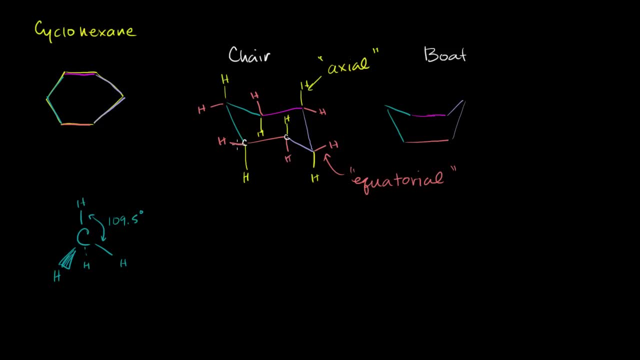 And the reason why they're called equatorial is, if you think about it- and it's sometimes hard to visualize- this bond right here is parallel to this bond right over there And this bond right over here is parallel to this. It's because equatorial bonds are parallel to some part of the 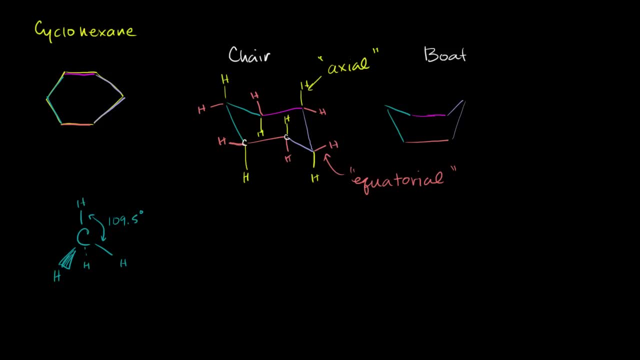 ring, So that one is parallel to that right over there. Actually, I could even color-coded that This. well, I don't want to use that same color. This is parallel to this And this is parallel to that, And we could do it for all the equatorial bonds. 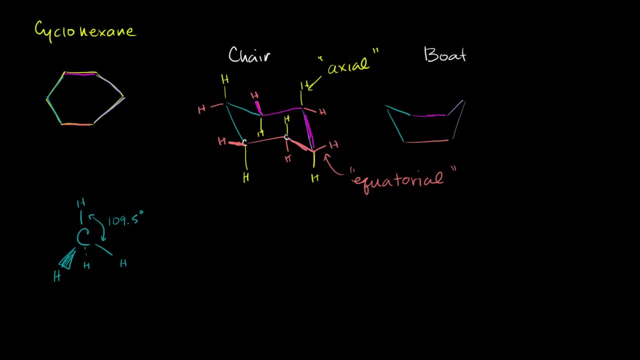 So, for example, I'm running out of colors here, so this right here is parallel to this, This and this and that over there, So we could keep doing it for all of them. I could do it for the other set right here. 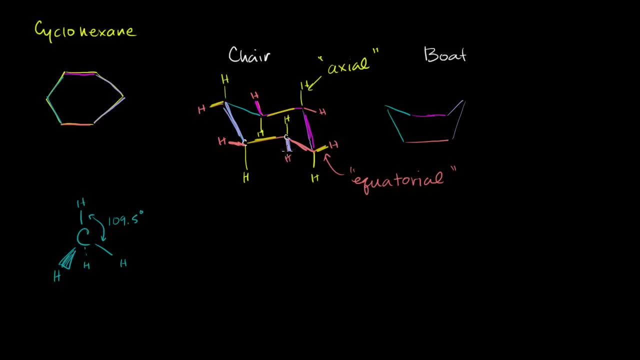 This guy right here is parallel to that guy over there. I didn't quite draw it like that, but hopefully it makes the idea clear And I'll do one more of these just to show what's parallel to what This bond is parallel to that. 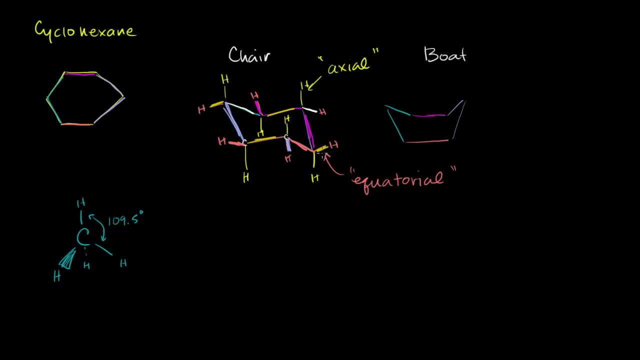 So the ones that are parallel to some part of the ring we're calling equatorial, And the ones that kind of jump out of the ring that aren't parallel to any other part of the ring, we're calling those axial. And the way I've drawn it here the axials are the ones 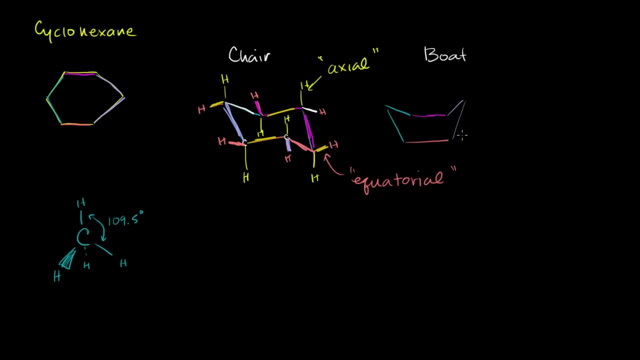 that point straight up and point straight down. We could do the same thing on a boat configuration. Now one question you might ask is: well, there's these two configurations. Both of these would result in tetrahedral-type shapes at each of the carbons. 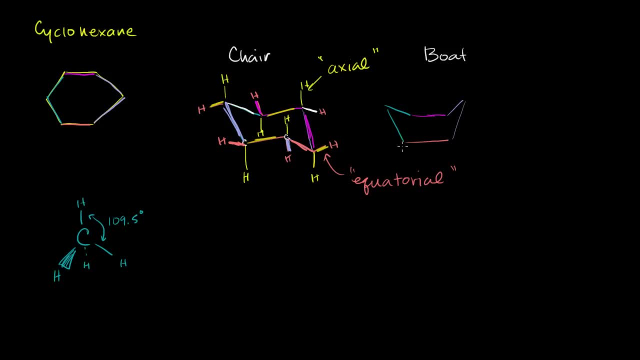 In fact, let me draw it for you. So this axial hydrogen is pointing straight down, This one is pointing straight down. Here this hydrogen is actually going to point straight down Because we've flipped it up And then over here you would have a hydrogen that points. 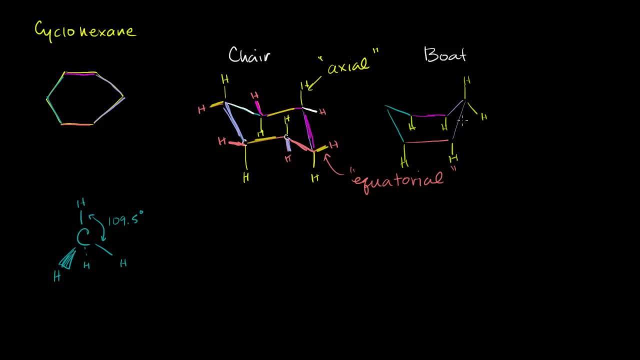 straight up and then one that's kind of pointing down. This gives a tripod there. To have the tripod over here you'll have to have a hydrogen that points a little bit like that. one that points a little bit like that, one that's pointing a little bit like 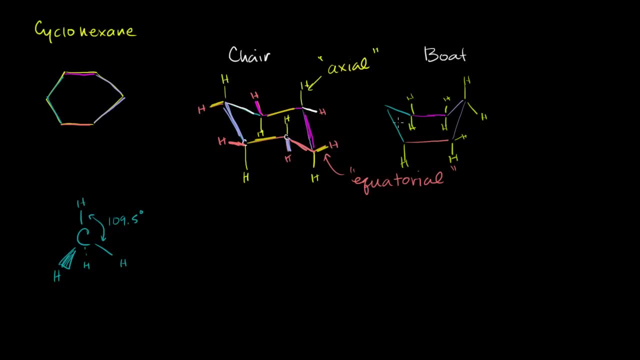 that along. Well, you can kind of view it along the same plane, as this guy would be parallel. It's hard to see it in this, but he would actually be parallel to that. This guy would be out like this, and then this guy would. 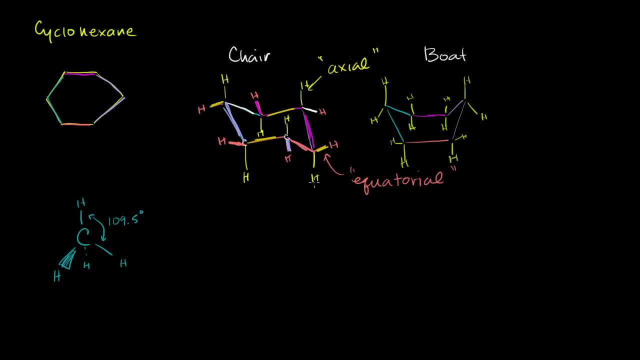 have an axial hydrogen And then he would have one equatorial one just like that, So you could draw the tripod shapes in either the chair or boat configuration. But one question is well, what's more stable? That's actually one of the main points of being able to. 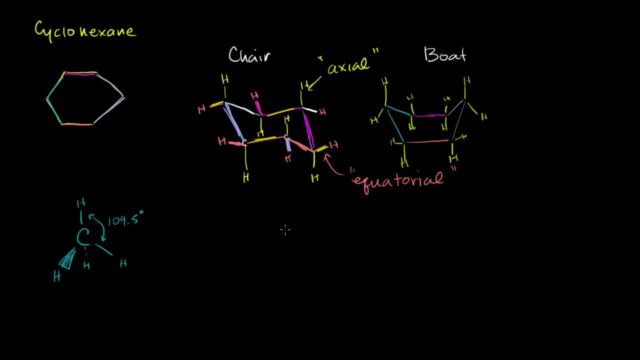 visually. think about the three-dimensional structure of any of these hydrocarbons or, in this case, cyclohexane. So in this situation, we know from past videos that all of these carbons with their hydrogens around them, these bonds, these have electron clouds around them. 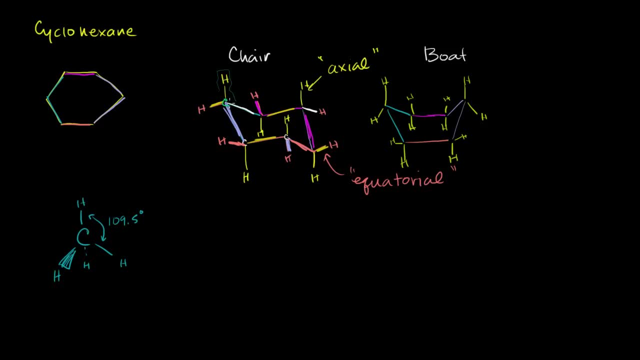 The electron clouds are negative, and so they want to get as far away from each other as possible. In this chair configuration you have this carbon up here. this carbon, the CH2, we could consider It, has two hydrogens and it's connected to. 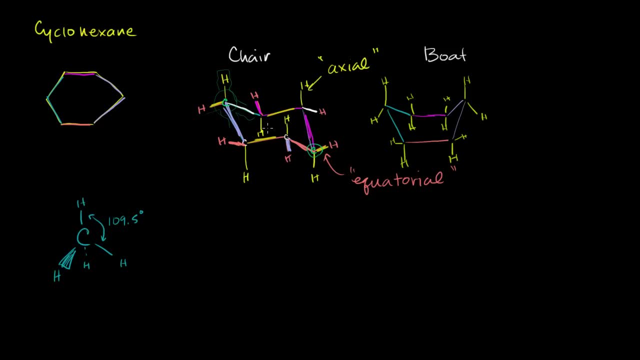 the rest of the ring. It's as far as possible from this CH2 as possible. So in that situation we have a lower potential energy or it is a more stable shape or more stable configuration In the boat configuration. this CH2 up here is much closer to. 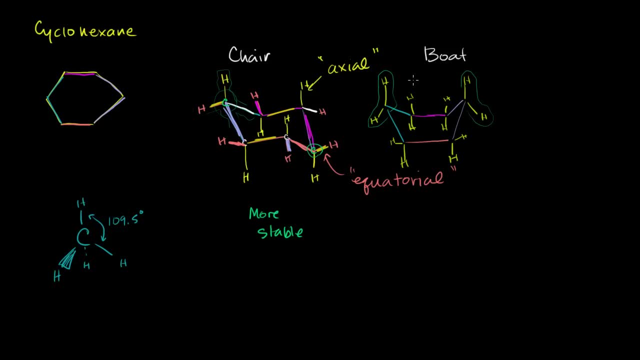 this CH2.. I mean, that's really the main difference between the two, And they want to get away from each other, They want to repel each other. So this one will have higher potential energy or it will be less stable. 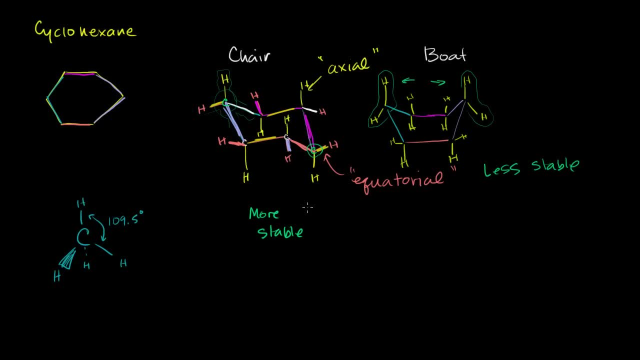 So this is just a starting point of how to visualize cyclic hydrocarbons, And we'll use this information in the next video to think a little bit more about, maybe, the different chair configurations that a molecule could have and what could be more stable. 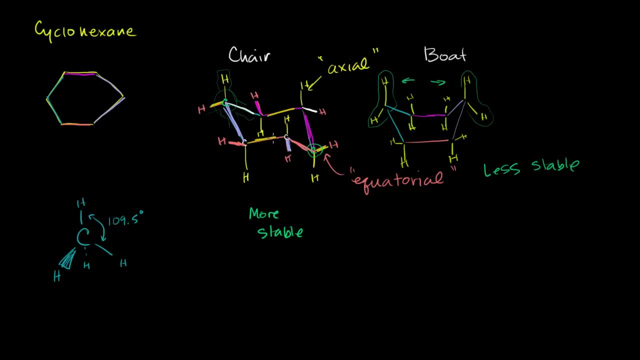 In this situation, in the case of just cyclohexane, the two chair configurations are equally stable, And let me just touch on that a second. So you have- well, I don't have to actually, let me see, I won't copy and paste it. 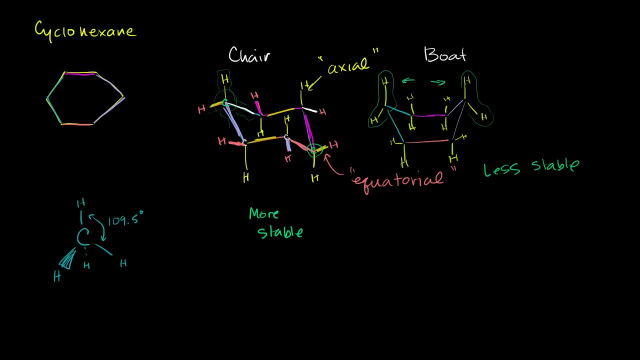 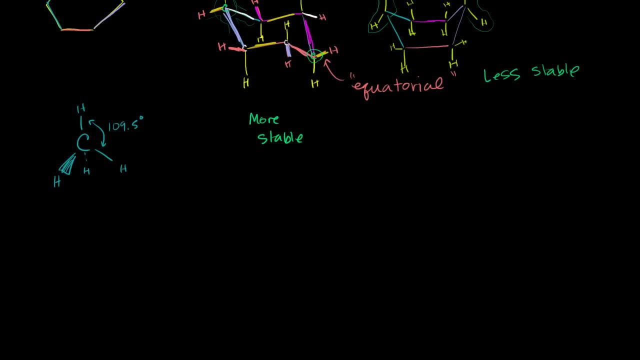 I'll just redraw the other chair configuration for this guy. Actually, let me just do it separately over here because I've made the colors here so confusing. Let me draw two. The same, The same cyclohexane, but in two different chair. 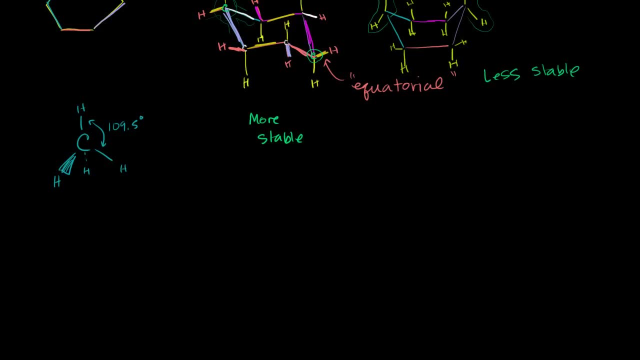 configurations that it could be equilibrium in, So you could have this one, You could have this one, So this could be one chair configuration, And I'll draw it like this, And then the same hydrocarbon could be, or the same cyclohexane could be, in equilibrium with this other. 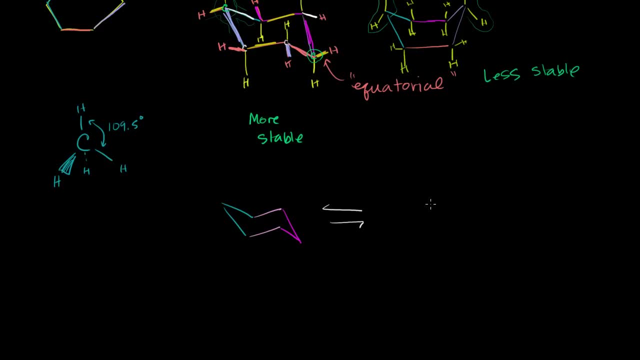 chair configuration. that looks like this. That looks like this: Let me have a little more space here. So it looks like this: Let me do the pink Goes up like that, like that, Let me make sure I'm. no, I want to do it actually. 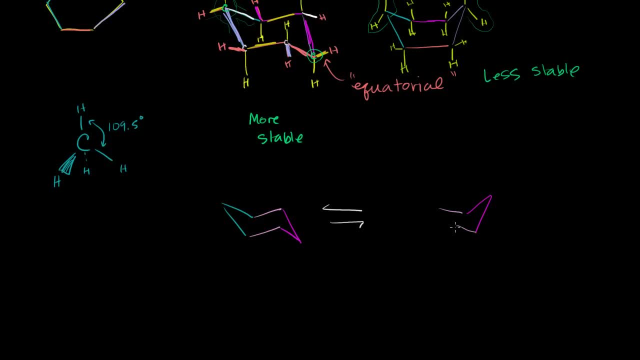 This pink guy goes like this, And then the blue guy is going to be just like this. So notice, in this situation, this carbon appears Here, is kind of at the top of the chair, And this carbon is at the bottom. And then they flipped. 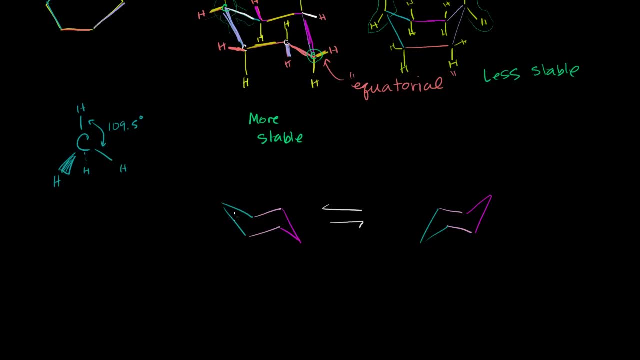 But these are equally stable configurations. But one thing to think about is all of the axial guys on this carbon here turned into equatorial on this carbon and vice versa on the two. Let me show it to you. Let me just draw the hydrogens on this carbon. 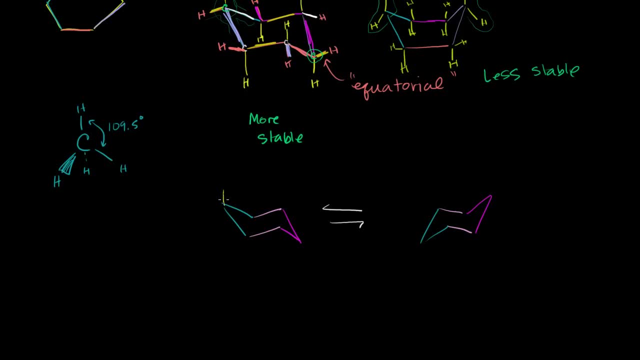 So if I were to draw this carbon's hydrogens, it has an axial hydrogen and has an equatorial hydrogen whose bond would be parallel to that right, Just like that. And this guy would have an equatorial hydrogen whose bond is parallel to actually both of these guys and an axial 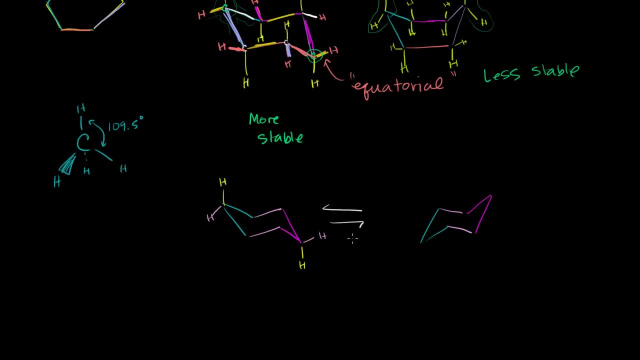 hydrogen. But when it flips- and I'm just drawing those guys' hydrogens- but when this structure flips like that, what happens? Well, this hydrogen over here goes into this position, And this yellow hydrogen over here goes into this position. 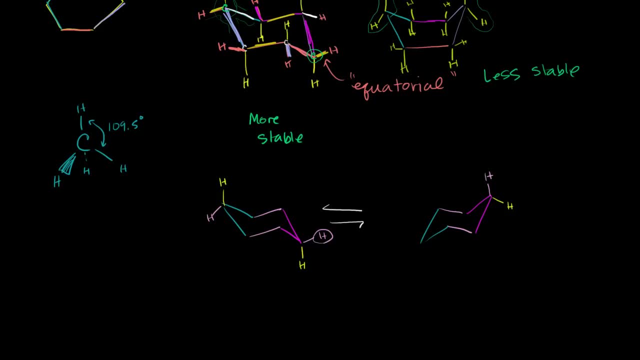 So over here it was equatorial and now it becomes axial. And the same argument can be made over here. This equatorial hydrogen, when this whole blue part flips down, now becomes axial. And this axial hydrogen when you flip it down. 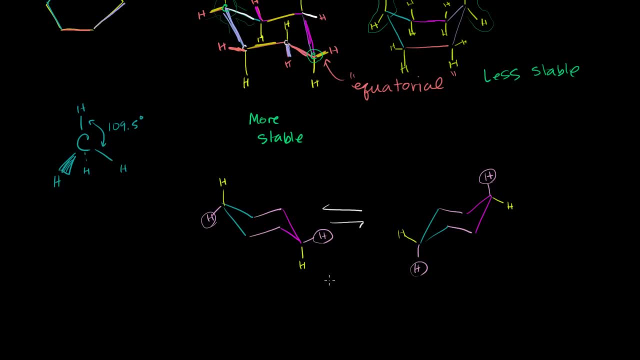 becomes equatorial, And you can actually do that for all of the hydrogens Over here. you have an axial hydrogen, Once you flip it. once you flip it, let's see you have an axial hydrogen, And then you have an equatorial hydrogen and an. 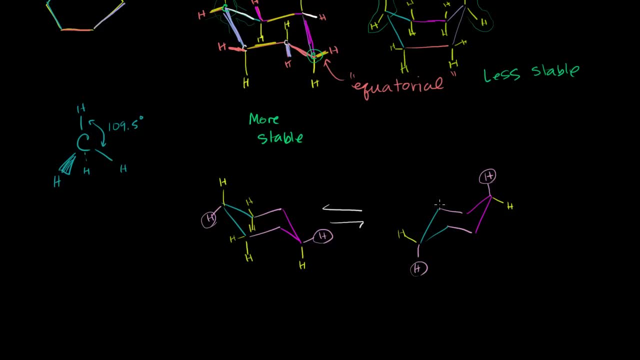 equatorial hydrogen. When you flip it, these two equatorial hydrogens become axial and then both of these guys become equatorial. So let me do that in yellow: Both of this guy and this guy become equatorial. So this and that become equatorial. 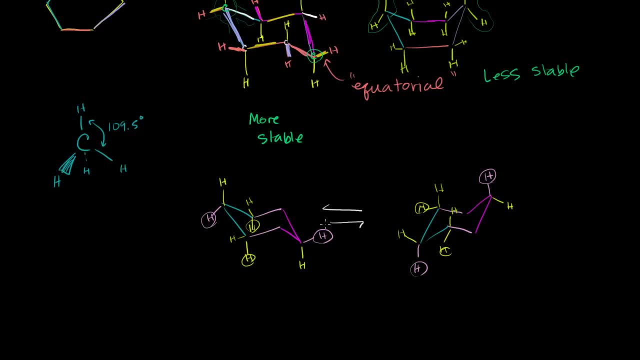 They become parallel to the other end, And you could do it for these two hydrogens as well. So that's another interesting to think about, and this is really just practical Practice on visualizing what's going on when we visualize these molecules in three dimensions. 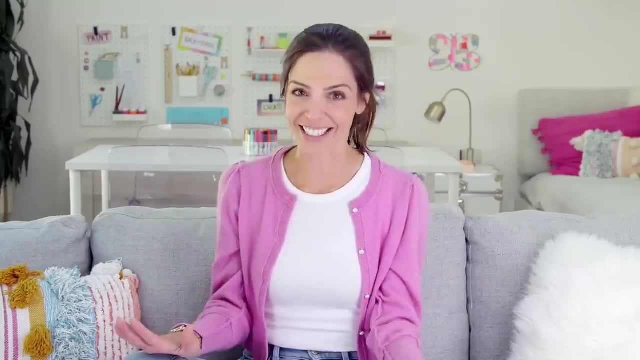 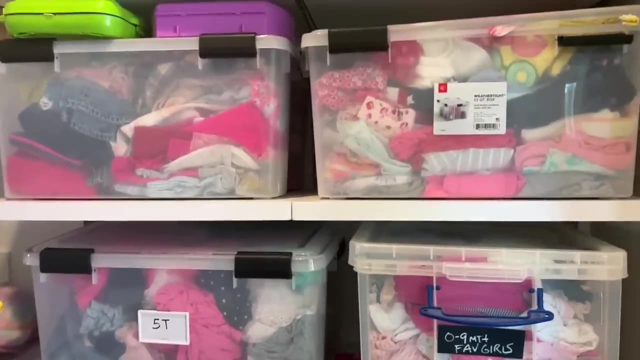 Hey guys, I am so excited- Actually I was not excited- to tackle Tess's closet. Look at the before. It's a bit of a hot mess. There was like four years of Presley stuff. We're down here A corner.